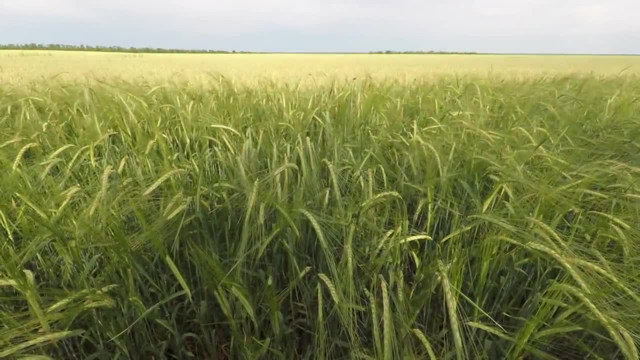 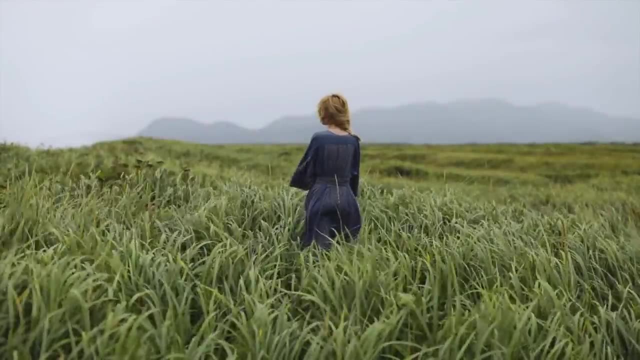 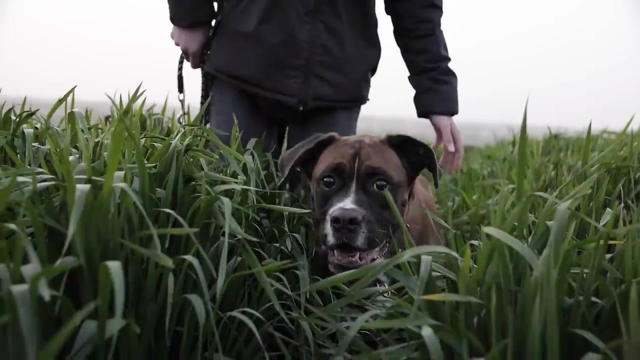 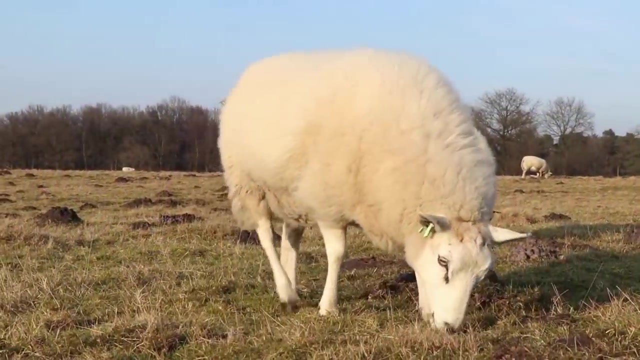 Grasses are adapted to hotter and drier climates than many other plants, like trees. There is a range of types. Some grow up to 7 feet tall, while others grow less than a foot tall. In the wintertime, the grasses die back to their roots. 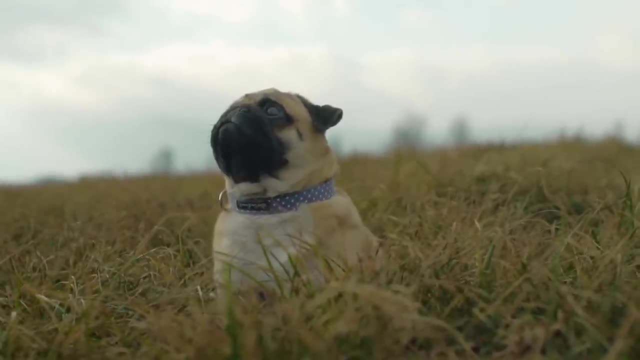 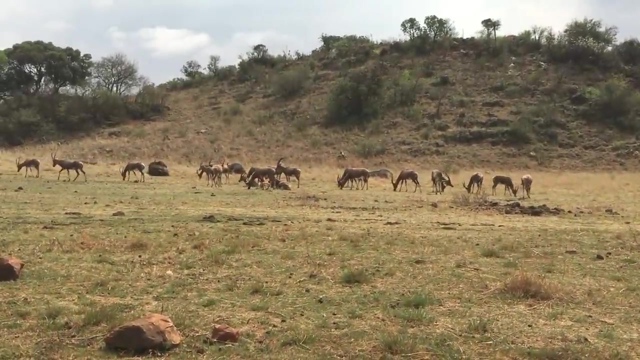 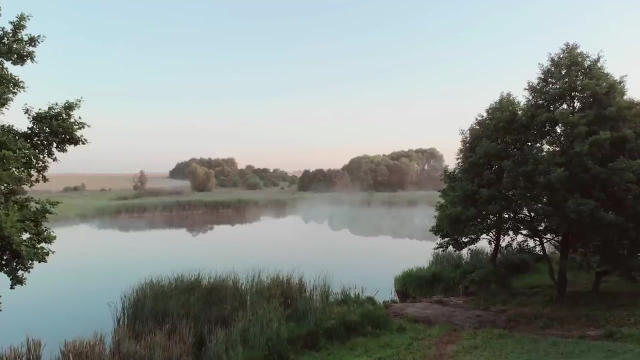 The dead leaves and soil on the ground protect the roots from the cold or dry conditions. The shrubs and trees are a great source of food for the grassland. The trees of the grasslands are fairly well spread apart and often found along streams and rivers. 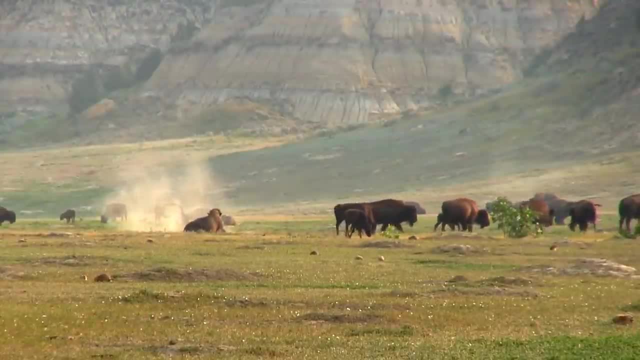 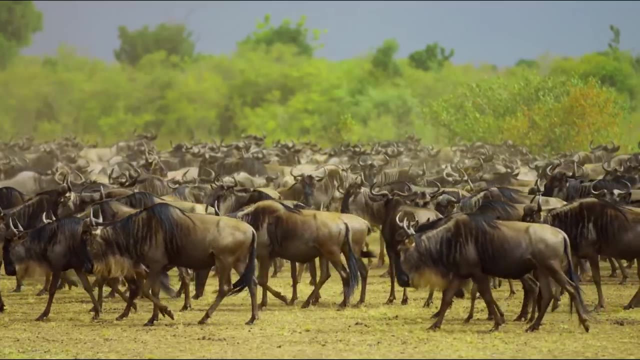 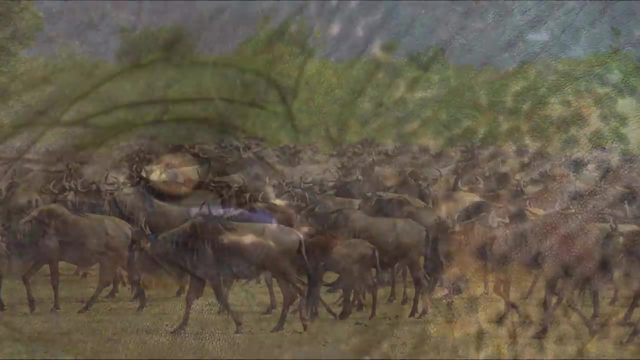 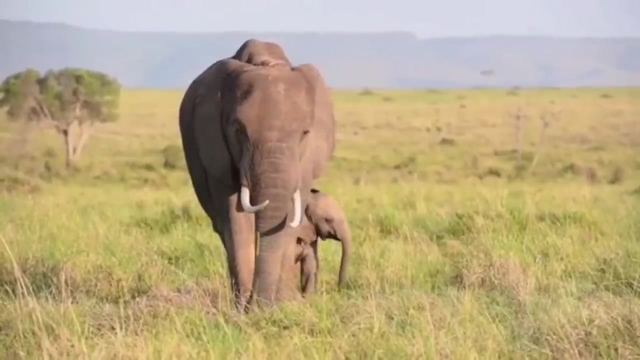 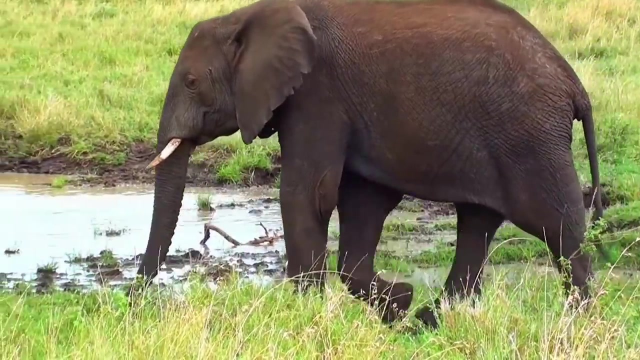 Animals that eat grass, like zebras, elephants and bison, help keep the areas from growing taller vegetation. They help reinforce the natural salinity of the earth by moving trees around迭 jego kanya, because they protect the soil away from our kerrios. 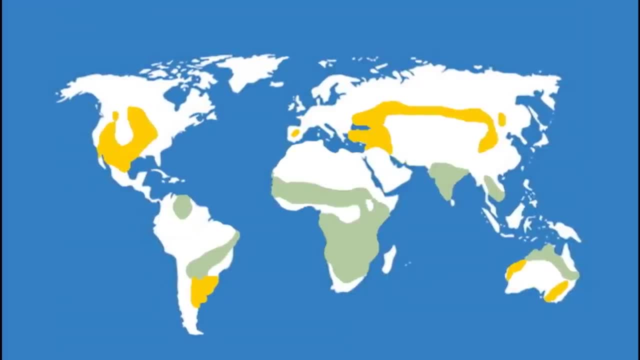 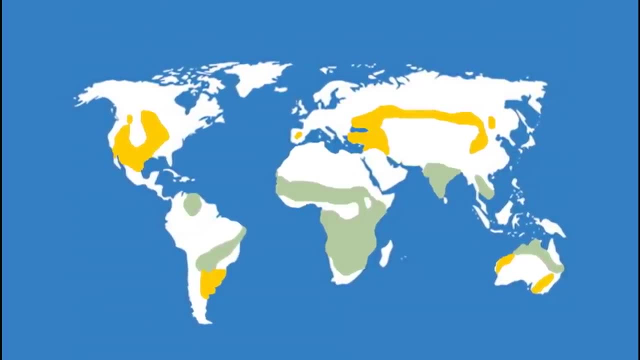 Elephants protect the savannah by crushing trees and shrubs and compacting the soil, which makes it easier for the grass to grow, but not the trees. are two main types of grasslands: Tropical grasslands, which are also called savannas. 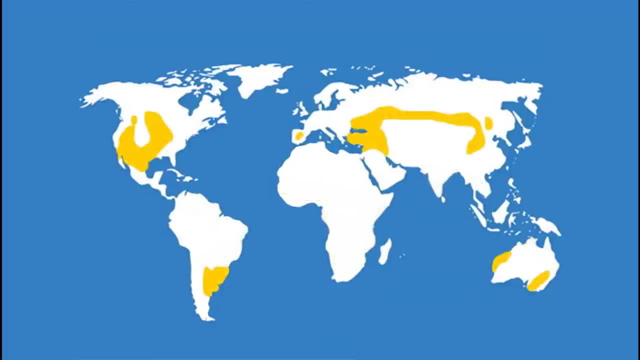 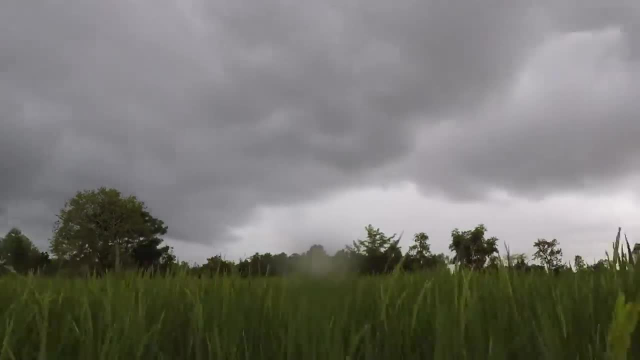 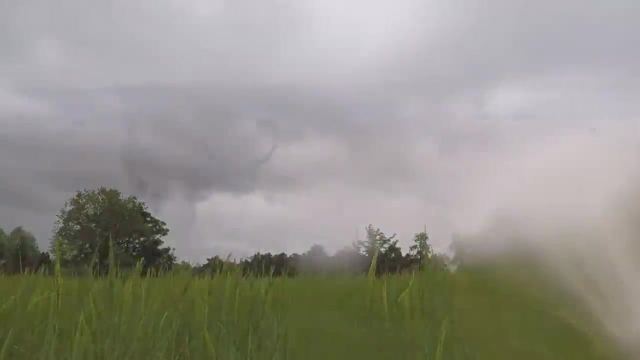 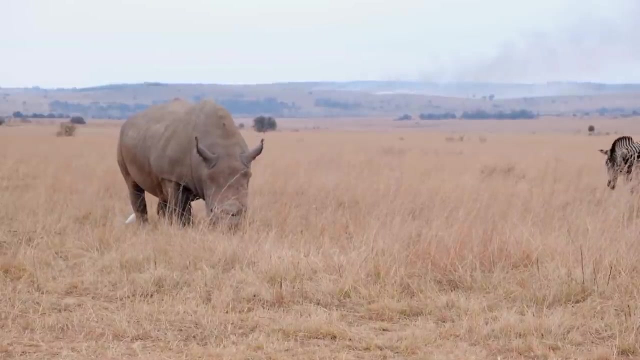 and temperate grasslands. Savannas have a warm climate with a rainy season and a dry season. Rainy seasons are usually just a few months out of the year. The long dry season prevents the growth of trees, because trees need more frequent rain. 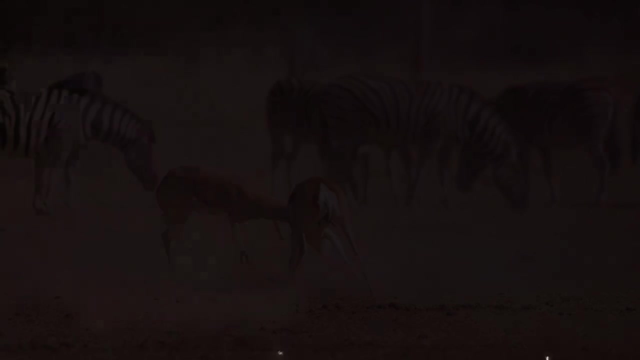 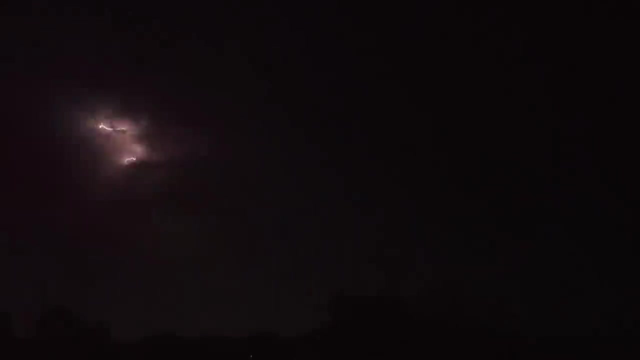 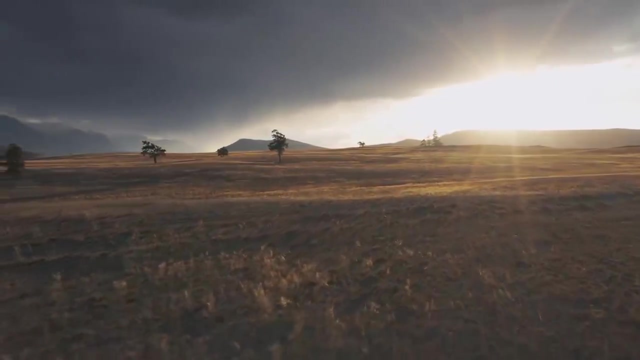 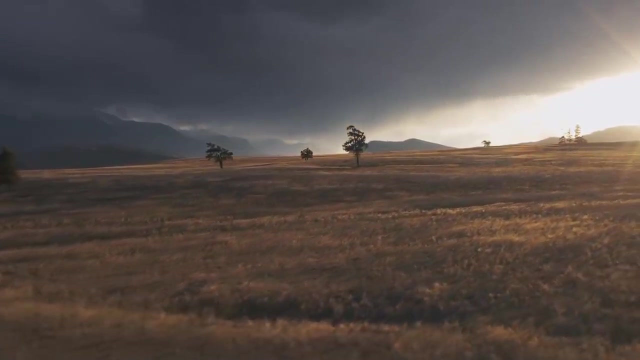 In October, many strong thunderstorms roll across the savannah, followed by strong dry winds. This begins the dry season. The dry season also prevents the growth of trees, because trees need more frequent rain. The dry season also prevents the growth of trees. The dry season also prevents the growth of trees. 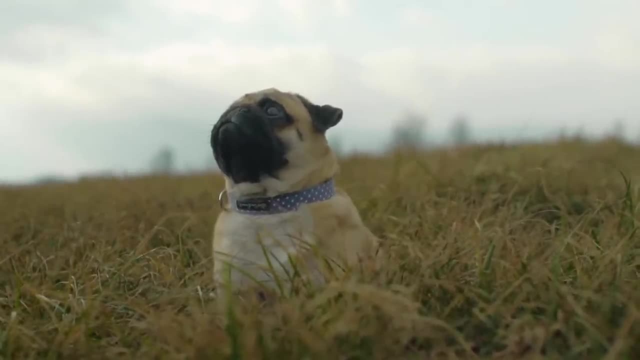 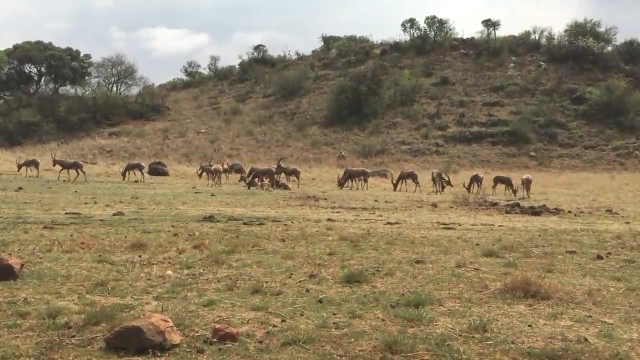 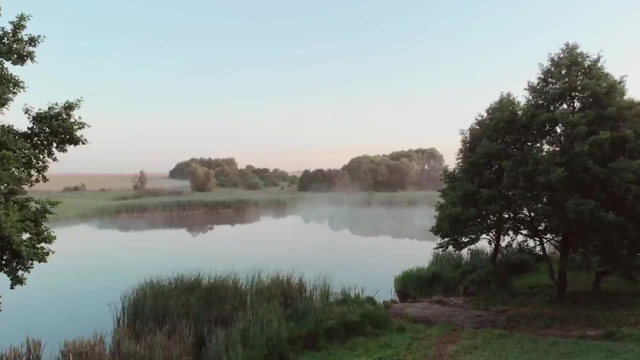 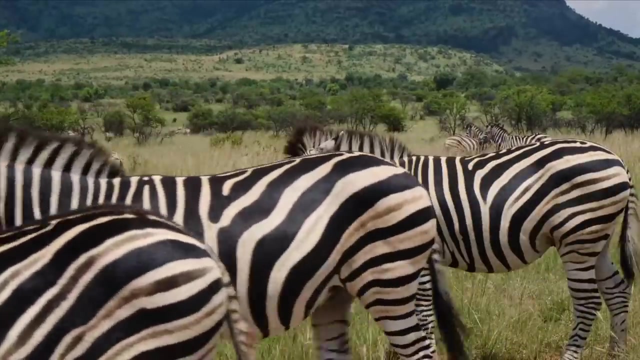 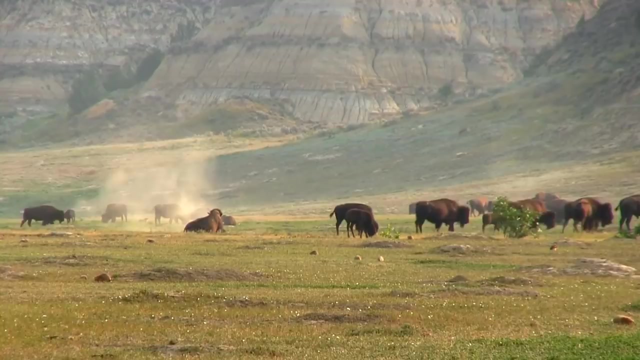 The dead leaves and soil on the ground protect the roots from the cold or dry conditions. The Shrubs and Trees- The trees of the grasslands are fairly well spread apart and often found along streams and rivers. Animals that eat grass, like zebras, elephants and bison, help keep the areas from growing taller vegetation. 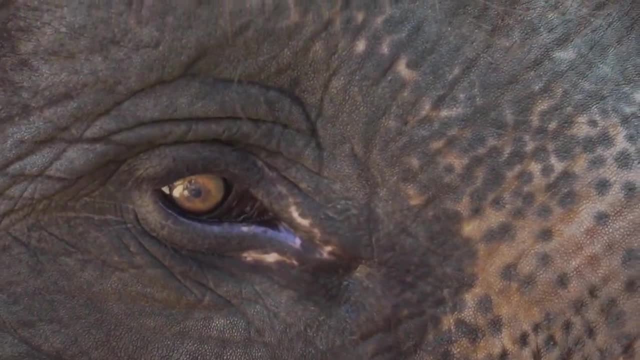 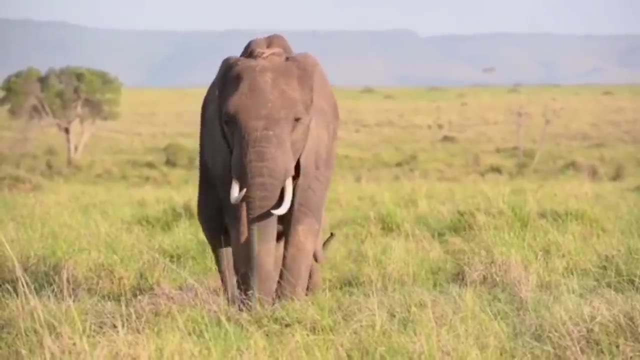 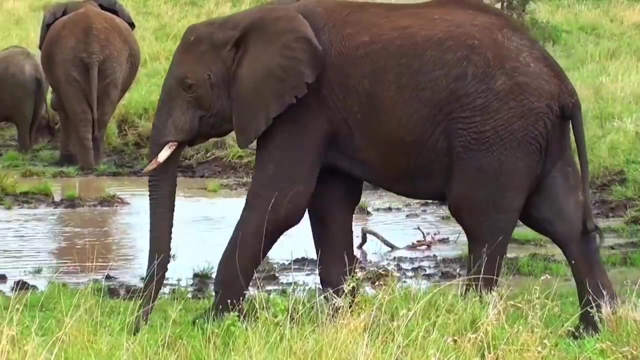 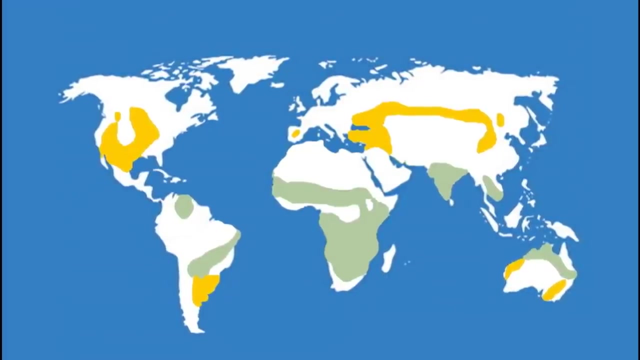 Elephants protect the savannah by crushing trees and shrubs and compacting the soil, which makes it easier for the grass to grow, but not the trees. The Grassland Biome. Grasslands are found on every continent except Antarctica. The Grassland Biome. 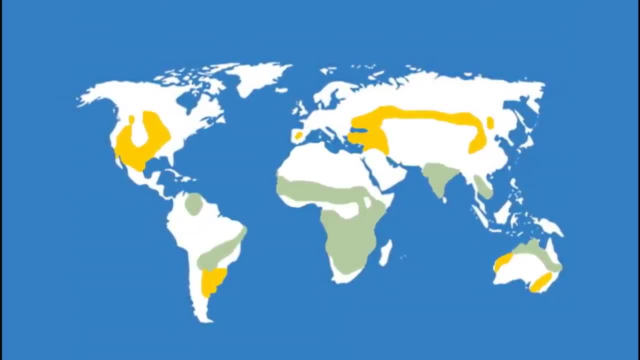 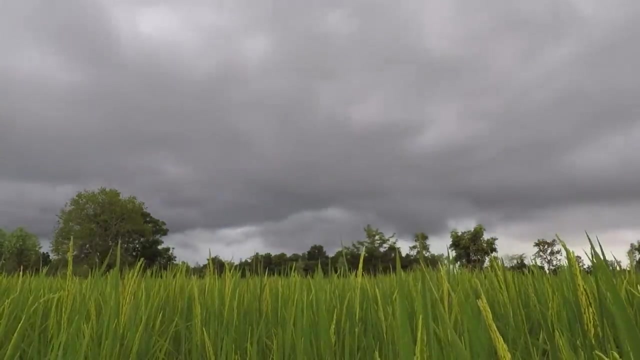 The Grassland Biome. There are two main types of grasslands: Tropical grasslands, which are also called savannas, and temperate grasslands. Savannas have a warm climate with a rainy season and a dry season. Rainy seasons are usually just a few months out of the year. The long dry season prevents the growth of trees, because trees need more frequent rain. In October, many strong thunderstorms roll across the savanna, followed by strong dry winds. This begins the dry season. The dry season also leads to wildfires, which kill taller vegetation. 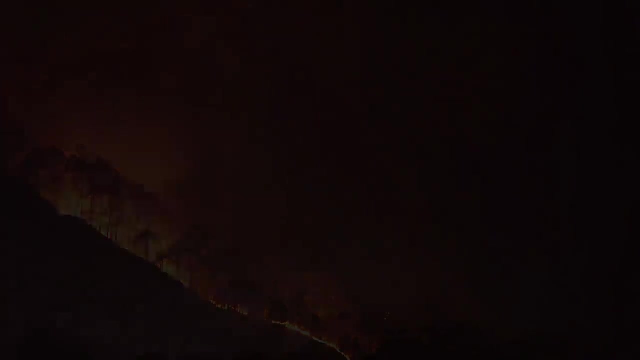 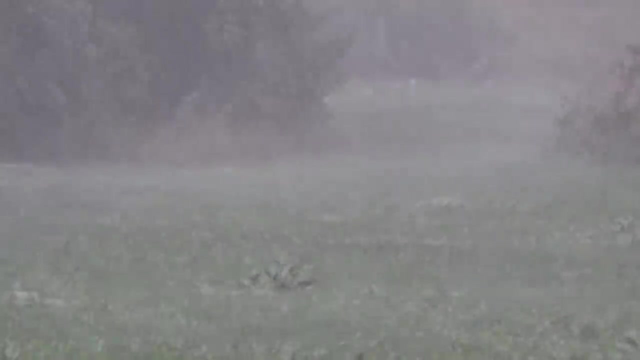 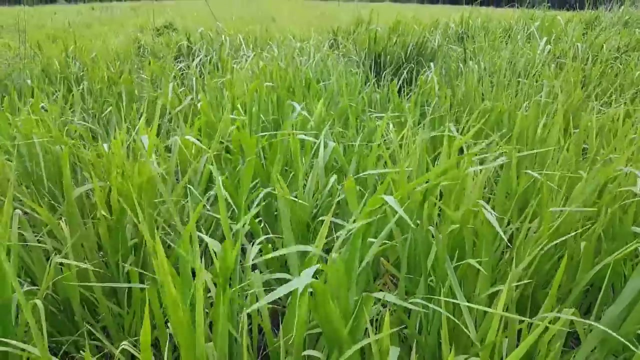 In March, the powerful thunderstorms return and the rains bring the savanna grasses back to life. In addition to grasses, wildflowers and wildflowers grow in the savanna. In addition to grasses, wildflowers and wildflowers grow in the savanna. 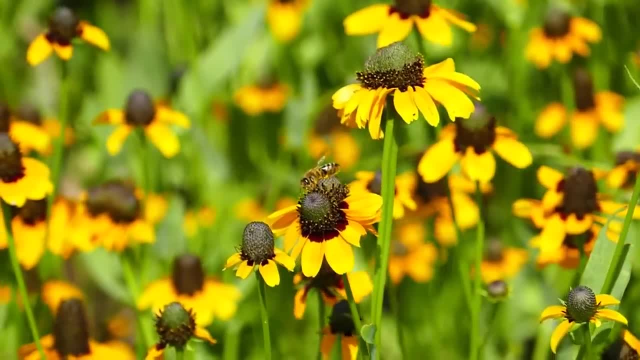 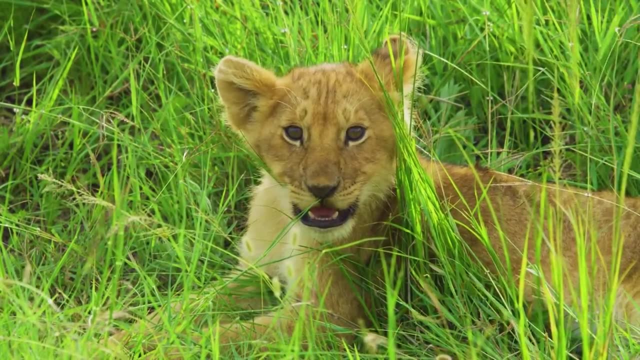 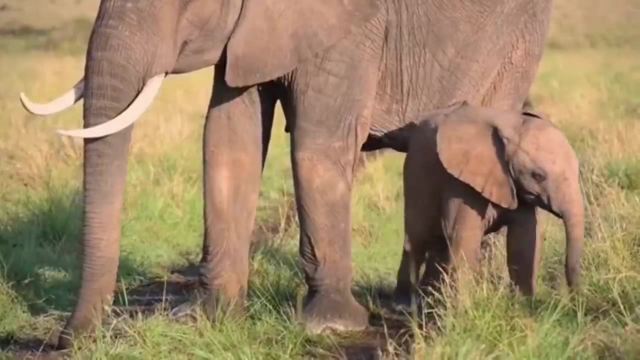 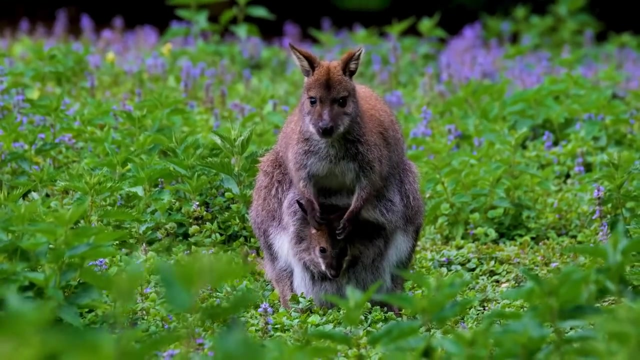 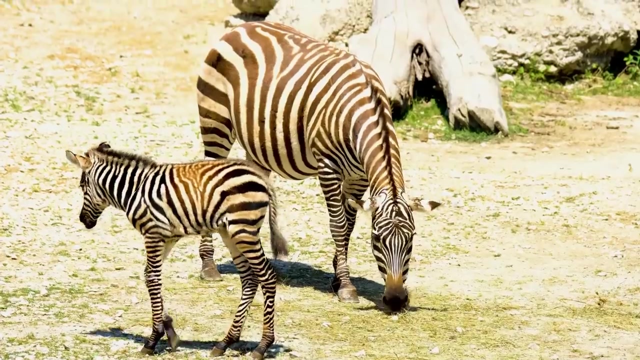 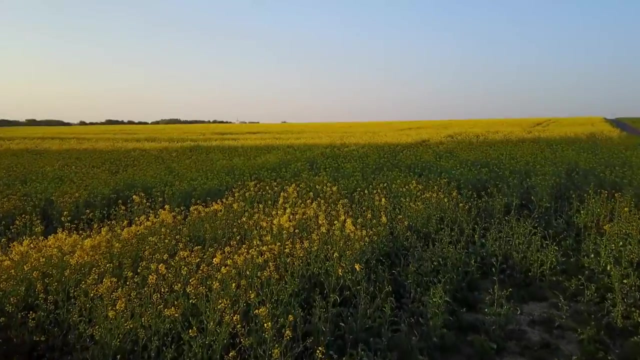 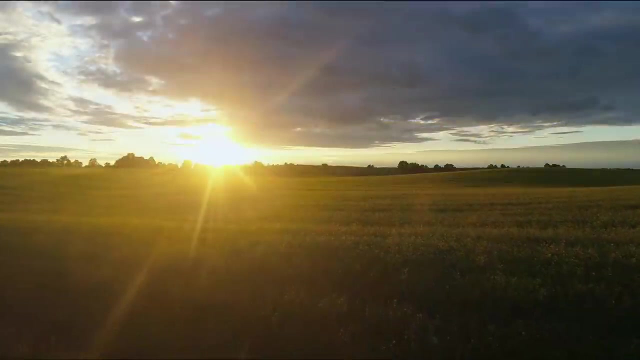 Small plants called forbs grow in the savannas. Along with this quick growth of plants, many baby animals are born. The temperate grasslands have richer soils with more nutrients. The temperate grasslands have richer soils with more nutrients, More variation in temperature between summer and winter. 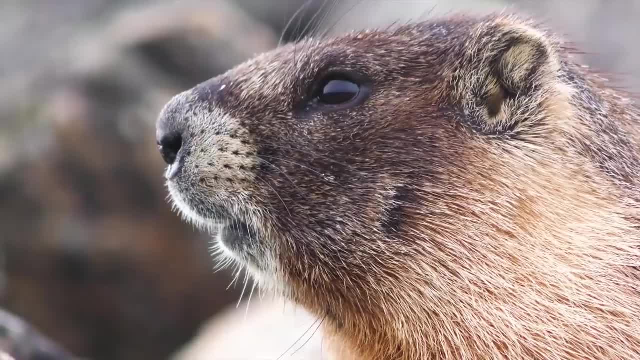 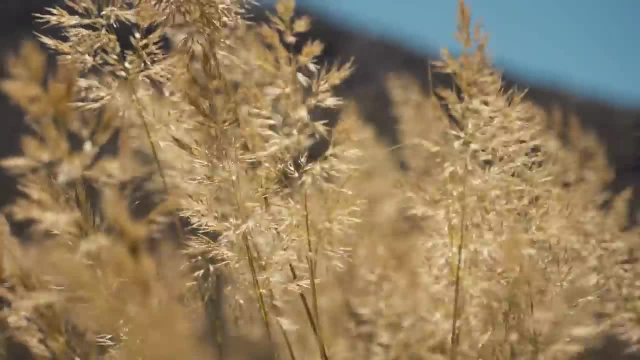 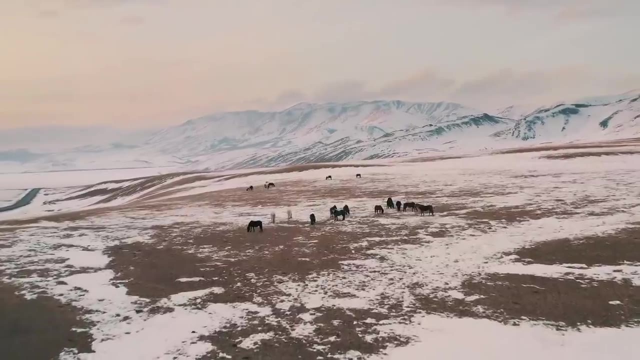 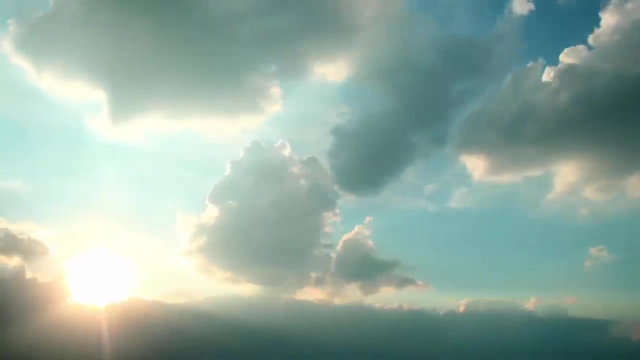 Summer temperatures can reach over 100 degrees fahrenheit or 38 degrees celsius. Summer temperatures can reach over 100 degrees fahrenheit or 38 degrees celsius, and winter temperatures can drop to minus 40 degrees. The temperate grasslands have less rainfall than in savannas. Rain comes in late spring and early summer. Temperate grasslands have grasses and wildflower plants, but no tall shrubs. Trees such as cottonwoods, oaks and willows grow along the rivers. Seasonal dry times, called drought, and occasional wildfires. 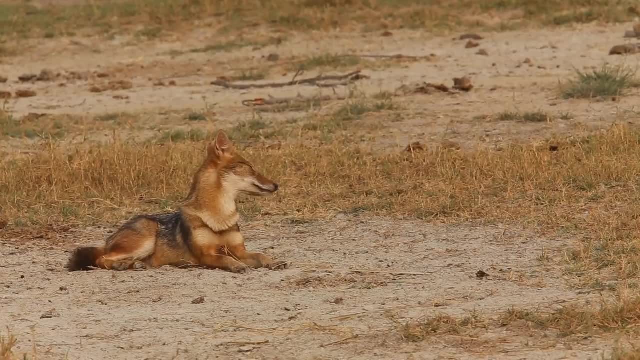 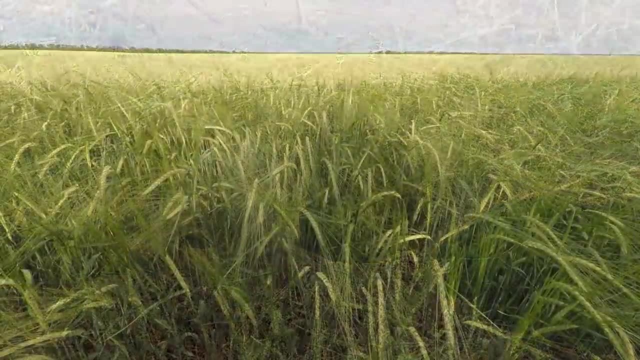 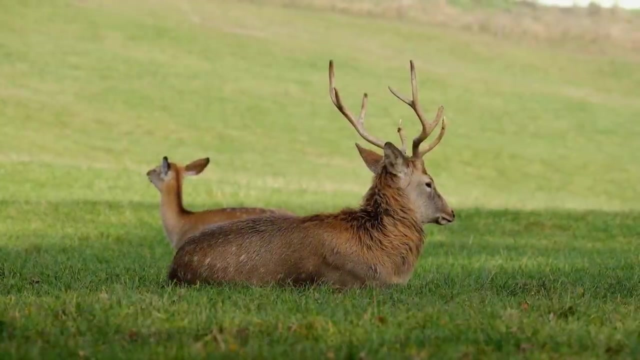 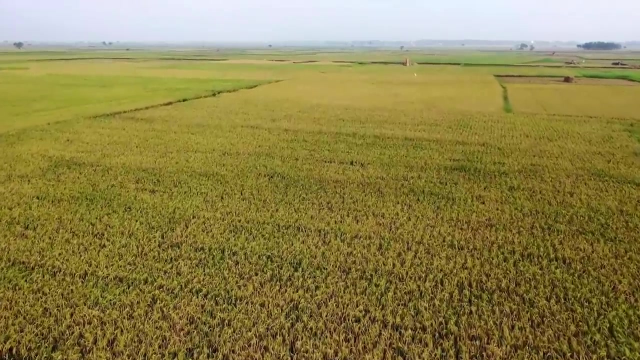 help to reduce the number of wildflowers. They help maintain this ecosystem. Temperate grasslands are divided into two kinds: Prairies have taller grasses, while steppes have shorter grasses. People have altered many of the temperate grasslands. 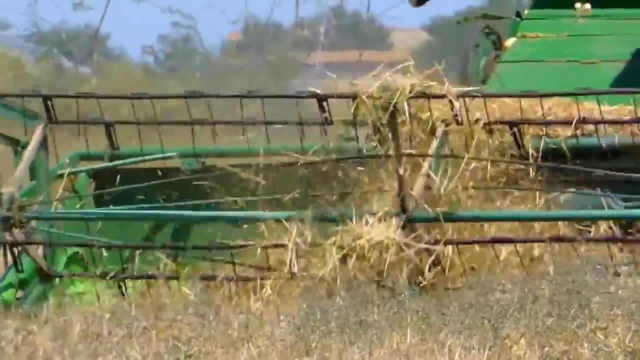 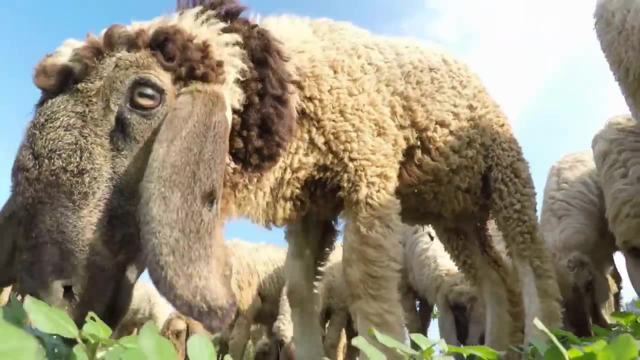 by converting them to fields for crops or grazing land for domestic animals like cattle and sheep. Temperate grasslands are divided into two kinds. Prairie grasslands are divided into two kinds. Prairie grasslands are divided into two kinds. 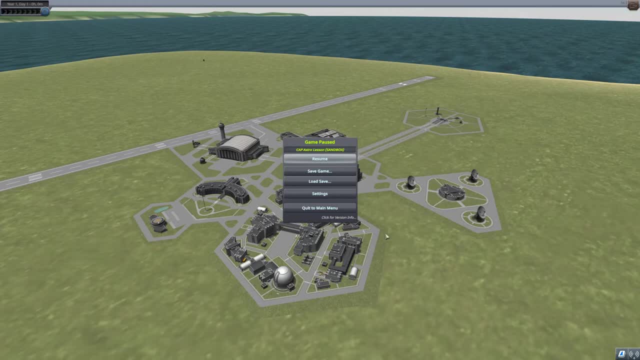 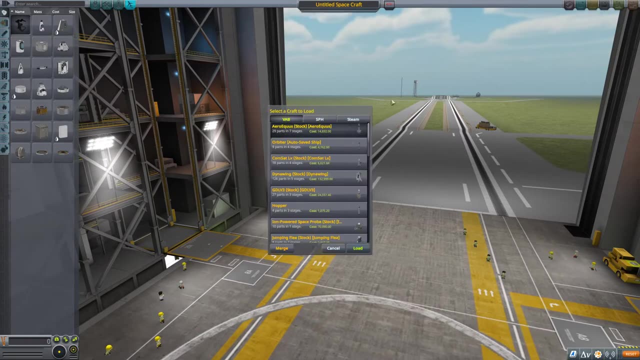 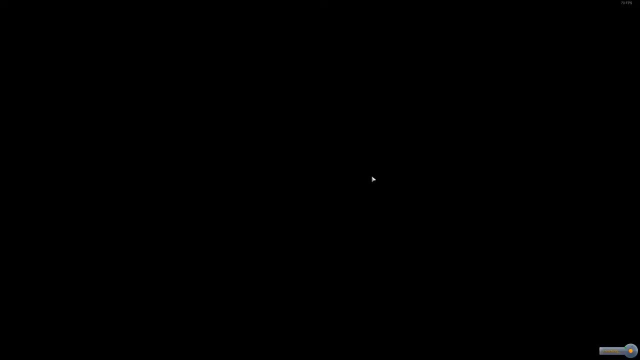 So today we will be using Kerbal Space Program and a little bit of math to explain how orbits work and how we build rockets to get there. So I'm just going to load up this rocket I have here and I'm going to set it up to launch right now. This will be a really simple demo and if you 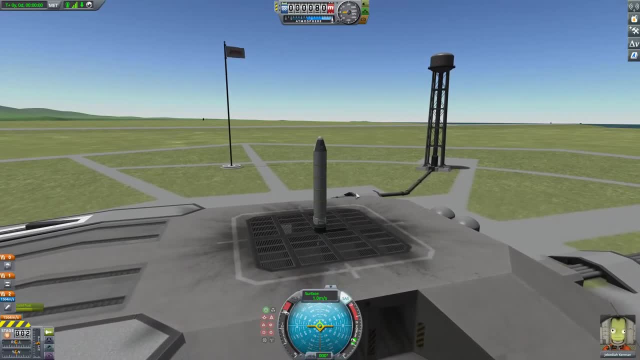 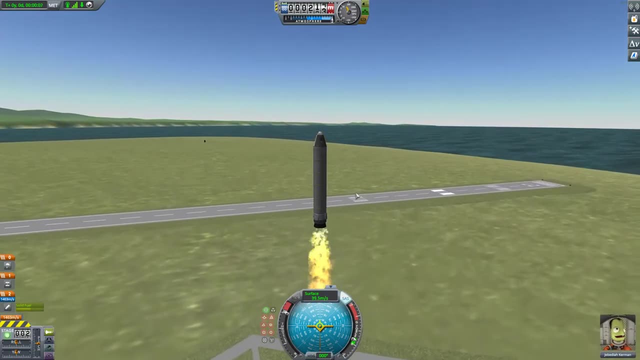 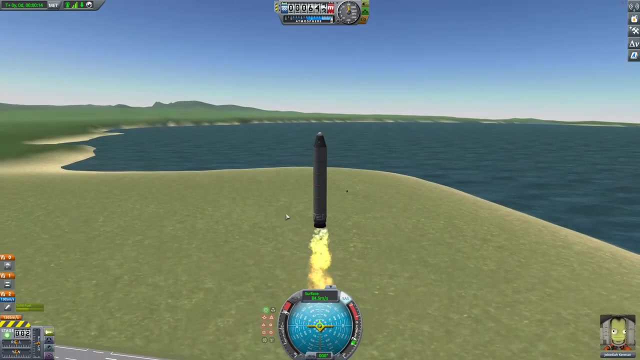 already know how to play Kerbal Space Program. this will be quite redundant for you, but I still hope that you can find it entertaining and perhaps maybe learn something new from it that you didn't before. But for today, we have one simple goal, and that goal is to get to orbit. 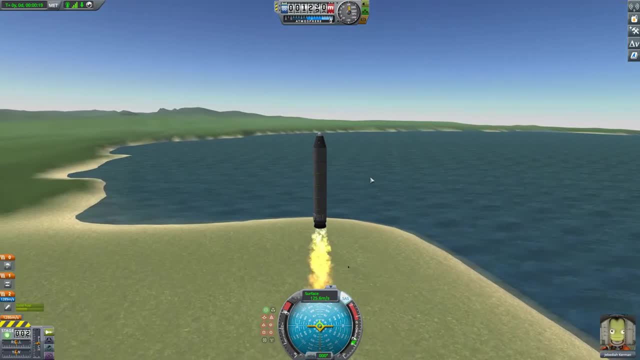 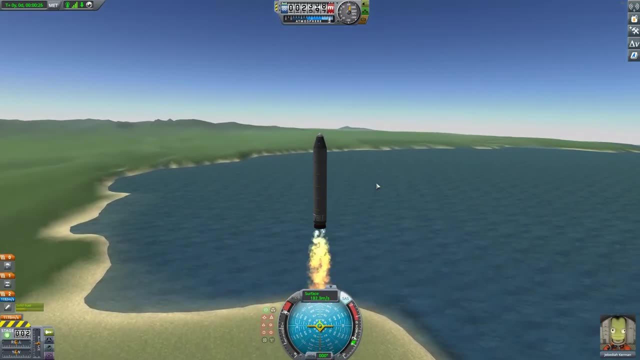 Let's find out if we do it. So what we have right here is a very small rocket, and some astute observers might say that it's not going to make it to orbit. Well, we're draining fuel pretty quickly here. We're almost at a quarter tank, as you can see in the